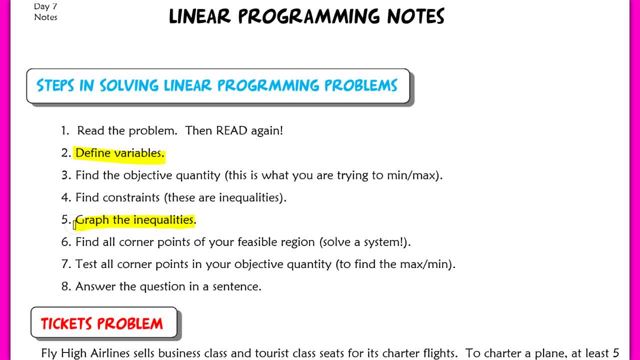 So next you graph them. So that's pretty straightforward. You've done this a lot. And then you're going to find your corner points for your feasible region- So that's that word that came up again before. So basically all you're doing when you find your corner points is solving a system. 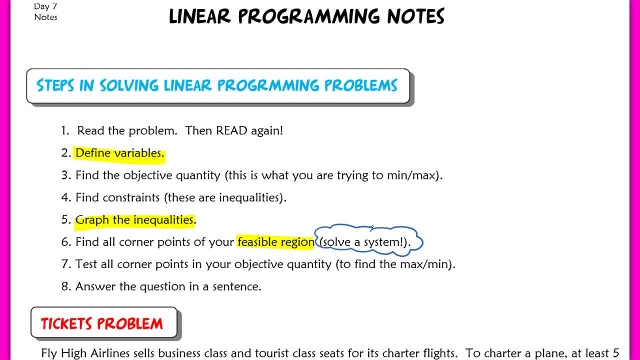 Again, just more skills that you've been doing in practice. Then, finally, you're going to test those corner points. So once you figure out what your corner points are, you will test those corner points inside your objective quantity to figure out which one produces the actual maximum or the minimum that you're looking for. 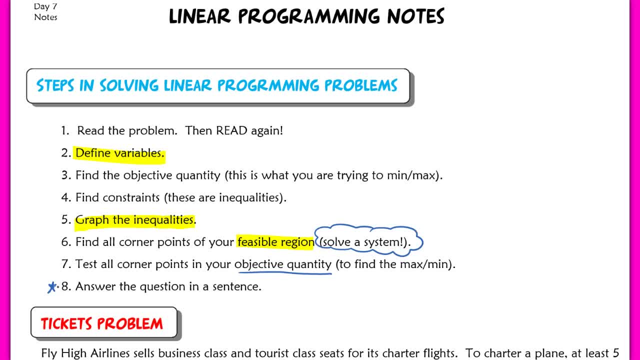 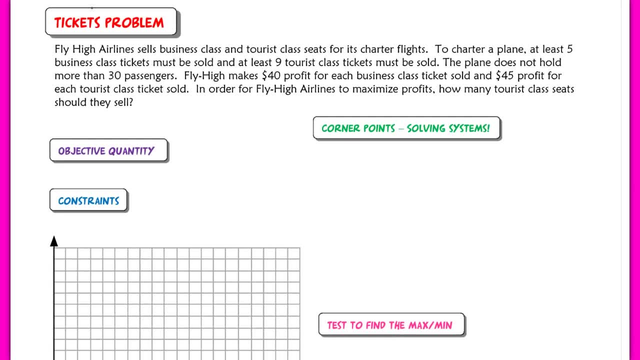 And then, finally, make sure you answer the actual question in a complete sentence. So let's begin. We have this tickets problem. Please pause the video right now and read this question. I want you to make sure you're familiar with all the parts, because I'm just going to go ahead and dive right into it. 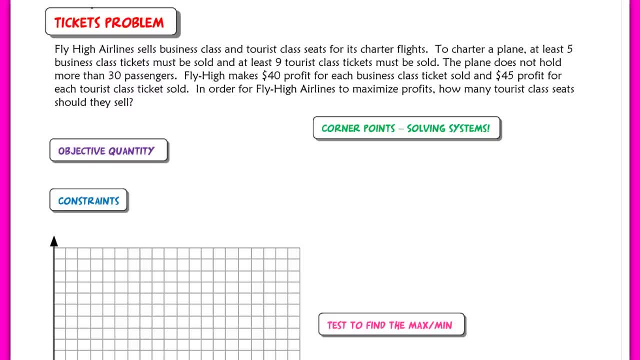 So let's begin. We have this tickets problem. Please pause the video right now and read this question. I want you to make sure you're familiar with all the parts, because I'm just going to go ahead and dive right into it. So let's begin. We have this tickets problem. 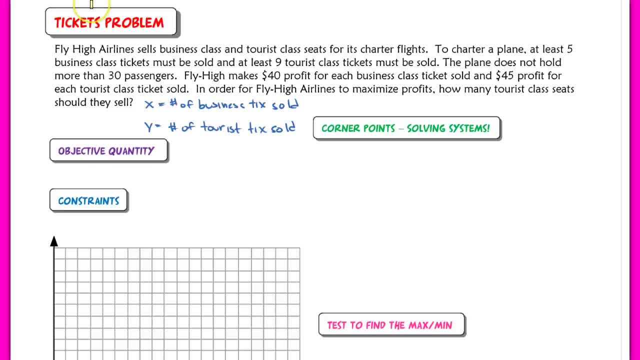 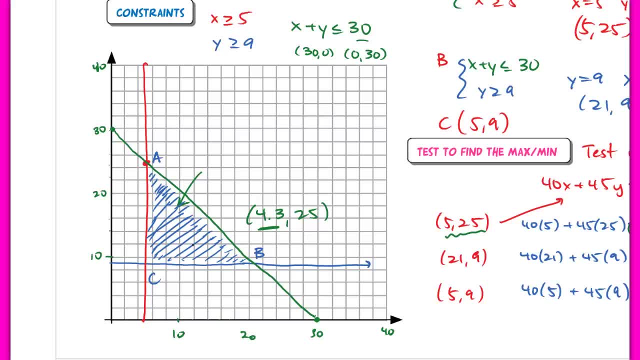 I want you to make sure you're familiar with all the parts, because I'm just going to go ahead and dive right into it, as opposed to the exact intersection. all right, Okay, the second problem here: this hamburger and hot dogs problem. 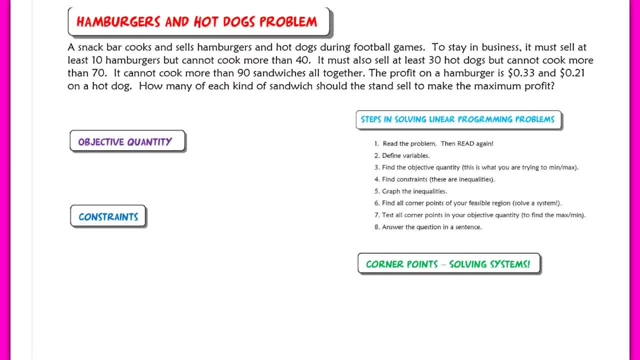 this is just for you to try this on your own tonight. I'm not going to check this necessarily, but you can check yourself with the key. I would definitely do this, though, just to get some extra practice and to make sure you understand what the steps are. So nice job and I'll see you in class tomorrow.